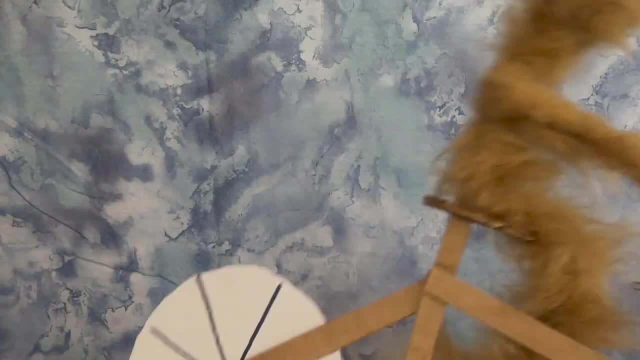 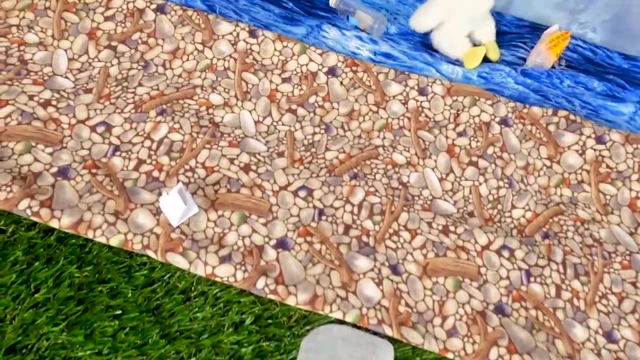 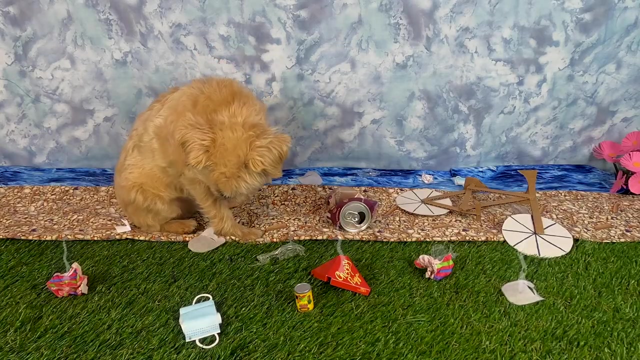 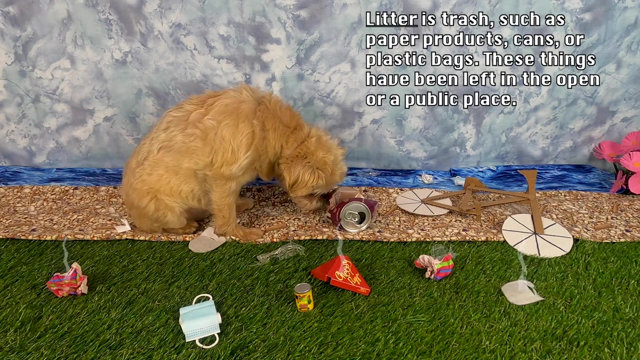 I tripped over this can. It's probably because this park is so full of litter. Litter is trash, such as paper products, cans or plastic bags. These things have been left in the open or a public place. Lucy, I saw you fall. 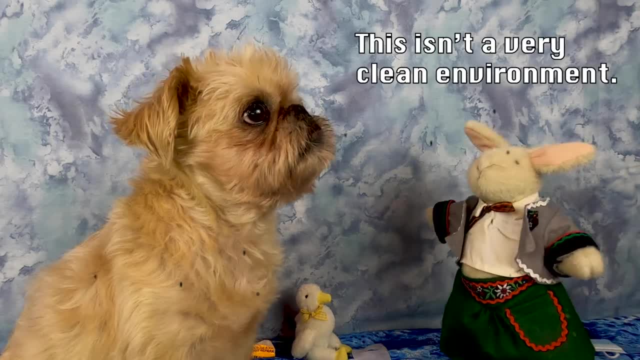 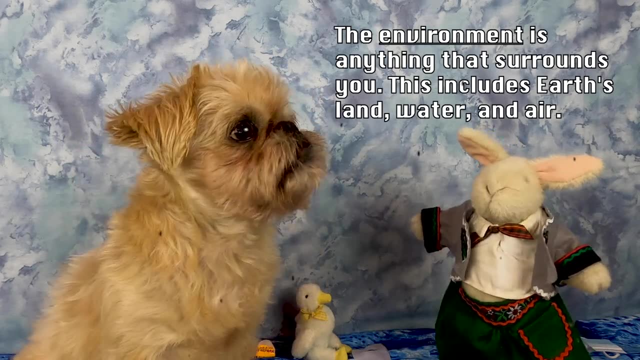 Are you okay? I'm okay. This isn't a very clean environment. The environment is anything that surrounds you. This includes earth's land, water and air. Litter, waste and other pollution can have a negative impact on soil water. 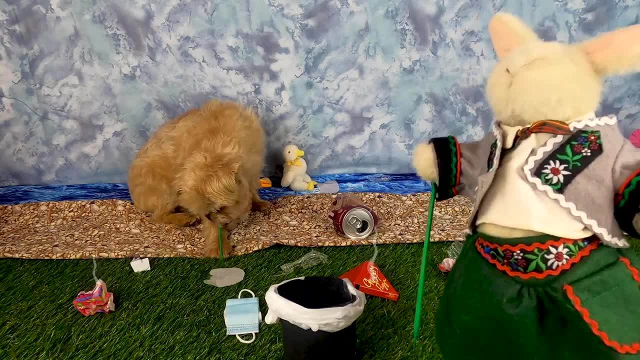 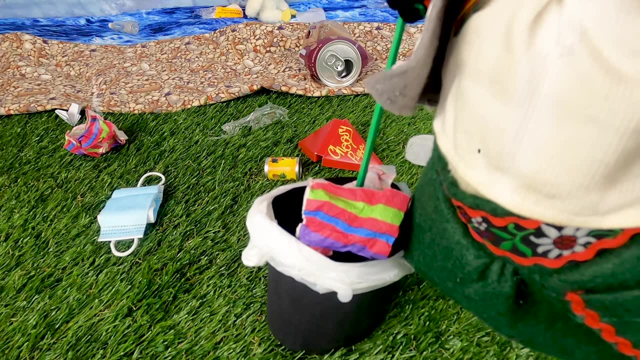 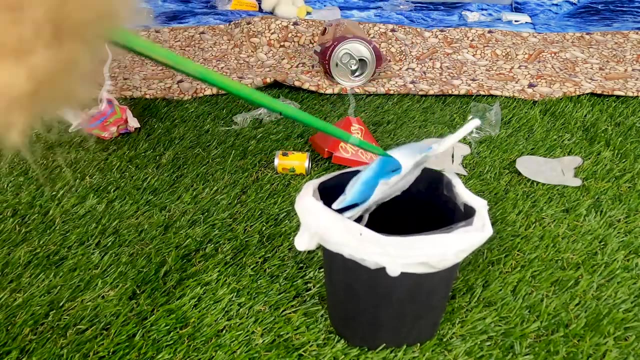 and the air quality. Lucy, that's not what I meant by reducing waste. We can use these trash pickers to grab the trash from around the ground and throw it away. Let's leave this place a litter cleaner than we found it. Waste is anything we throw away or get rid of. 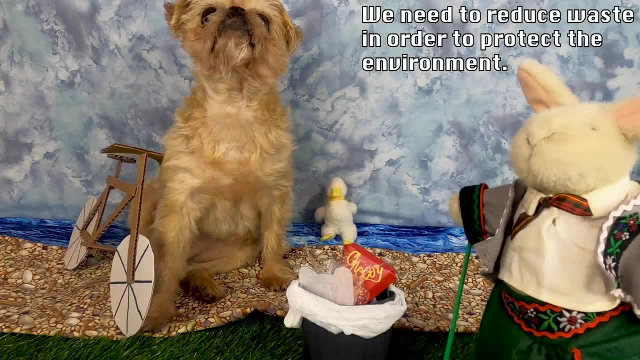 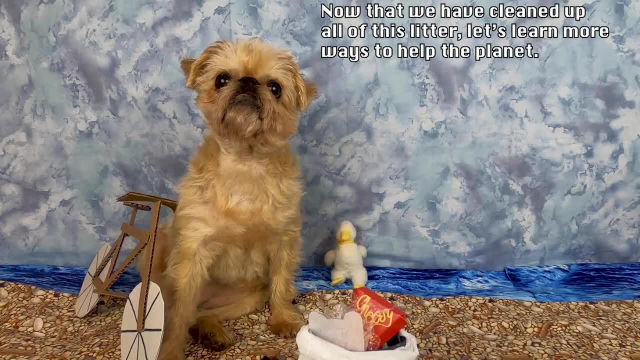 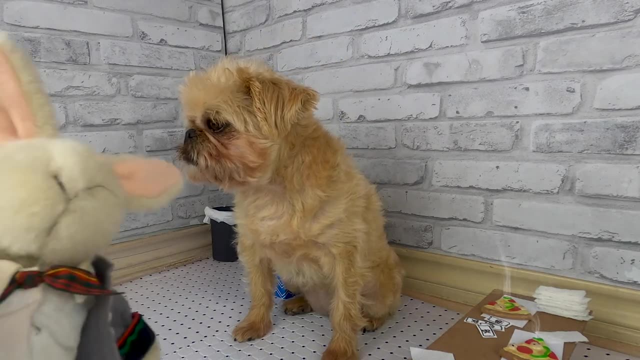 that doesn't get used. We need to reduce waste in order to protect the environment. Now that we have cleaned up all of this litter, let's learn more about ways to help the planet. I love school lunch. Lucy, did you forget what reducing means? 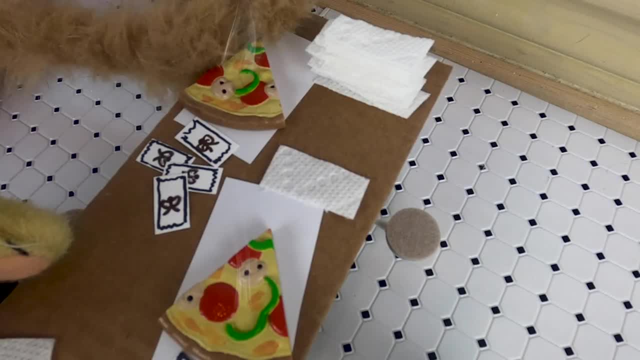 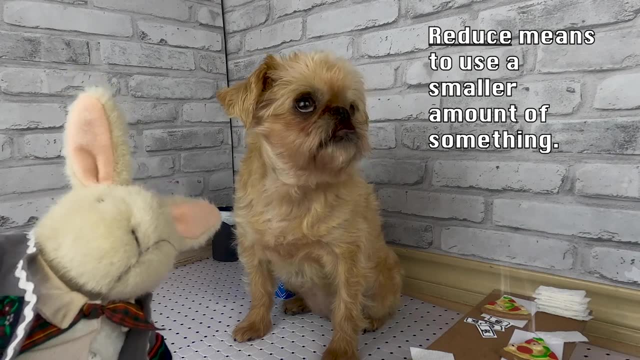 What? Why did you grab so many napkins and pretzels? I don't know, I didn't even think about it, I just grabbed them. Reduce means to use a smaller amount of something. When you use less, you waste less. 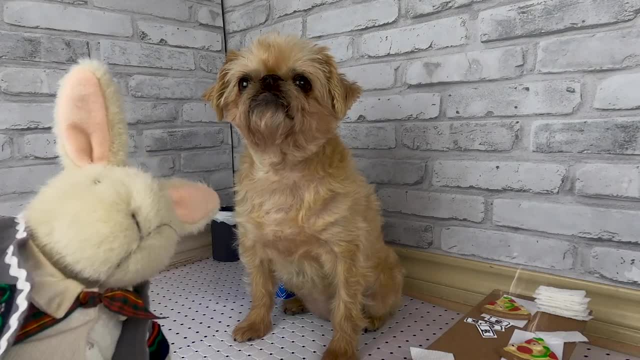 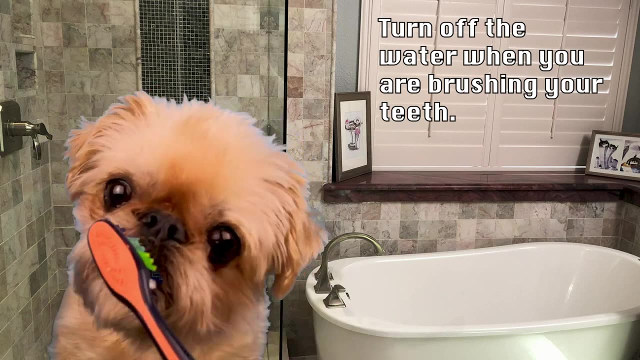 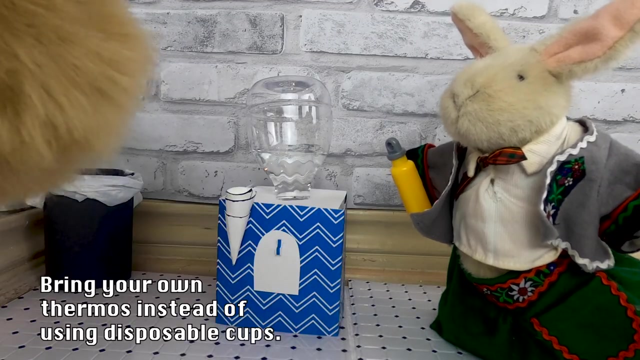 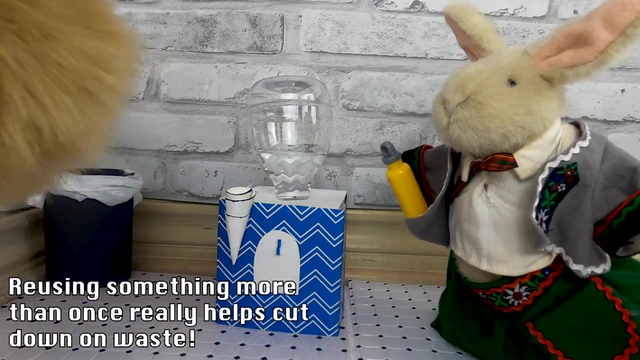 What are other things that you can use less of? I can think of one. Turn off the water when you are brushing your teeth. Bring your own thermos instead of using disposable cups. This is a great way to reduce and reuse. Reusing something more than once really helps cut down on waste.